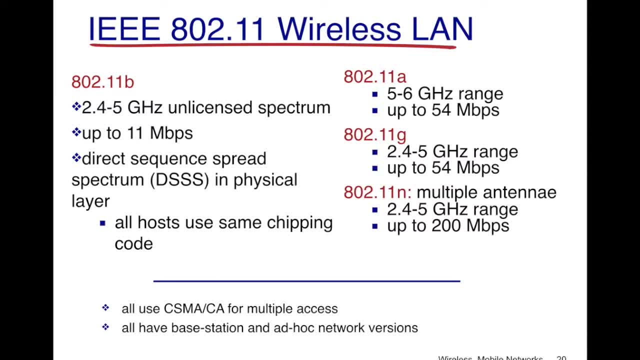 typically as standards. the newer standards offer more speeds than the previous ones. For example, A2.11b only offered up to 11 megabits per second, whereas A2.11n, which use multiple antennas, provides up to 200 megabits per second. Now, one thing that is common across all these different 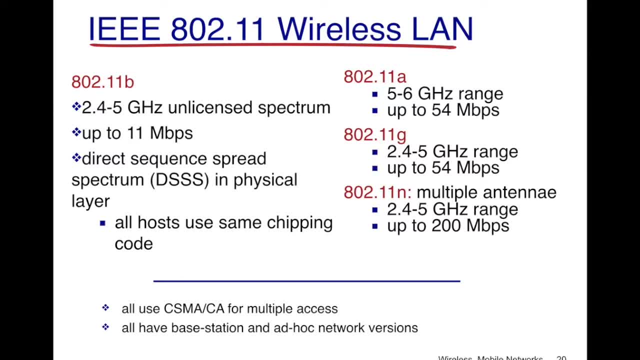 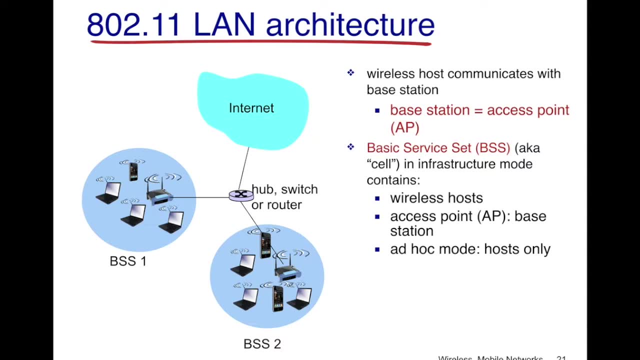 technologies is that they all use CSMA CA for multiple access and they all have base station and ad-hoc mode versions. Now CSMA CA may not make so much sense to you at this present moment, but we'll discuss this later in this video. Now the 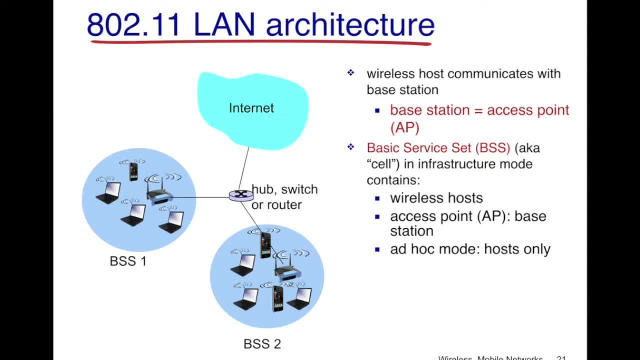 A2.11 architecture. let's talk more about that. So first we have the wireless host, which are your typical smartphones or smartphones. Now the wireless host, which are your typical smartphones or Wi-Fi, which connect to the base station. Now the base station in Wi-Fi network is 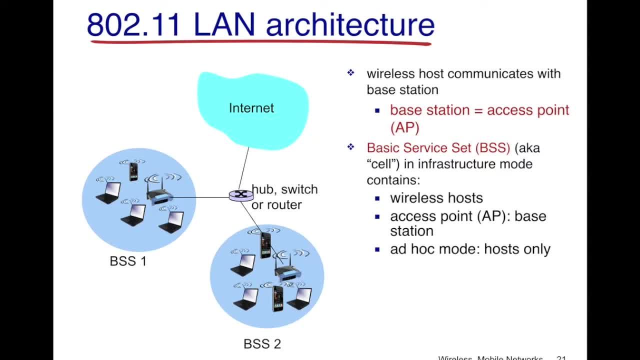 the access point. Now what we have is a basic service set, or BSS. It is also known as the cell in infrastructure mode, and what it contains is basically the wireless host- your smartphones, laptops, any other device which connects to your access point using the Wi-Fi network- and then the access point. 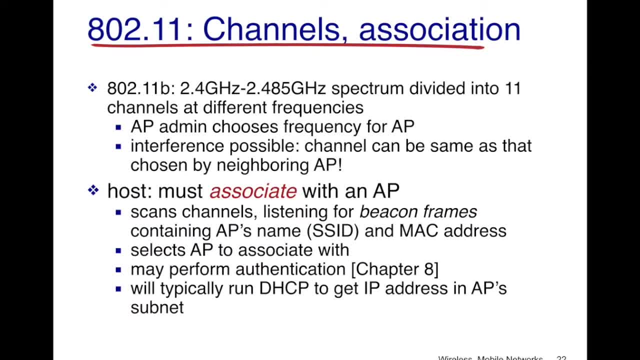 itself. Now the next component of an A2.11 network are the different channels and how the different hosts associated, associated with the access point, using these channels. Now I'll talk to you about A2.11b, though it's an older standard, but it's much of the things that I discussed today are also. 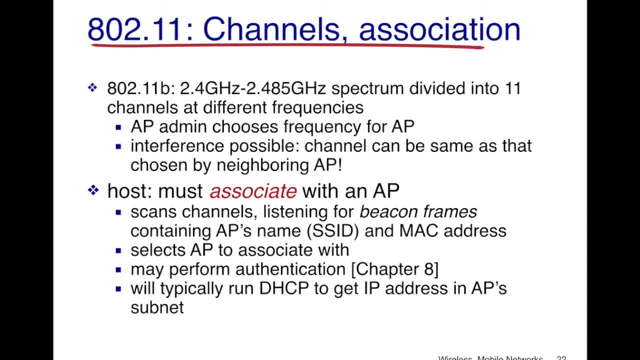 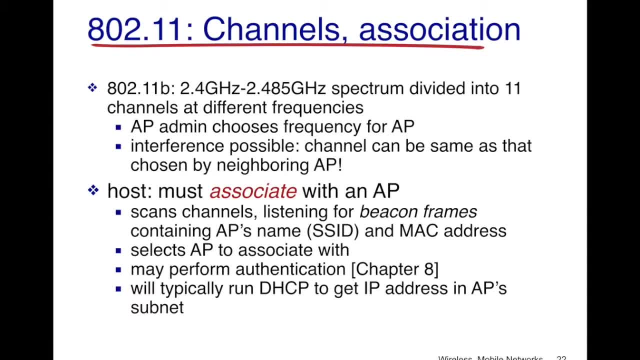 divided into these 11 channels. Now, if you're an AP admin or the AP, what the AP admin has to do is to choose the frequency to which this particular AP will be tuned into. Now, the way an admin chooses these different frequencies for the different access points in a building are to choose these channels. 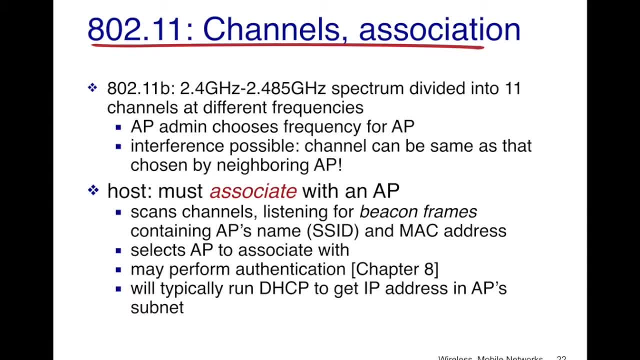 such that neighboring access points are have less, as less- interference as possible. Now, if you're a host which is a laptop or a smartphone, it has to connect with one of these access points. Now, if you, as soon as you enter the network- by you I mean the host- what it does is it? 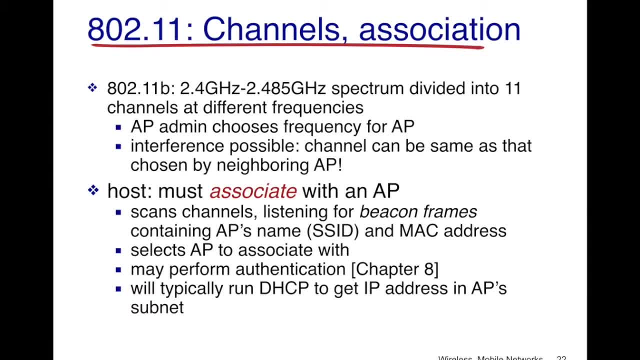 scans these channels and it listens for some beacon frames to understand if there is an access point nearby. Now these beacon frames, what they contain are the access points name, which is the SSID and the MAC address. Now, when a host enters into this Wi-Fi jungle, it 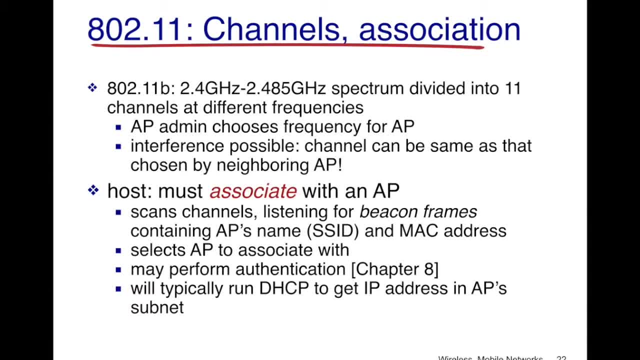 might actually receive a bunch of beacon frames from different access points. Now, once it receives all these beacons, what the host must do is it must choose the access point with which it has to associate with. Now this access point may require some kind of authentication, and we'll talk about authentication in a 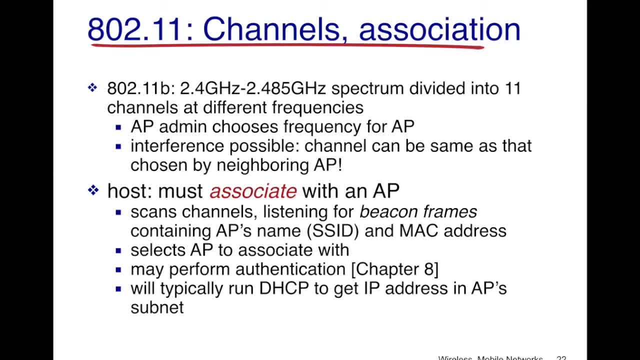 bunch later videos the host has been authenticated. the view usually what the access point does is it wants dhcp and if you recollect from previous videos, dhcp is used to get an ip address and then the host can get connected to this access point or is in the access point subnet and it can send packets to the 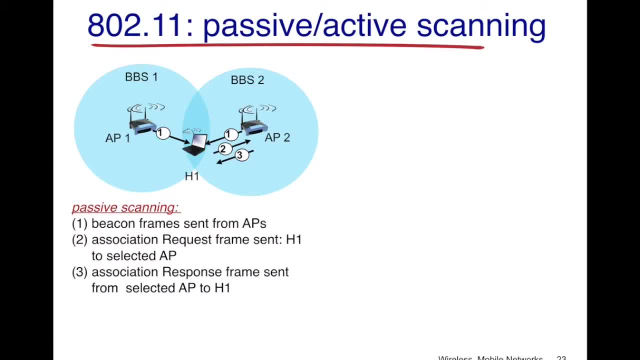 greater internet. so now let's see how a host actually connects to an access point. so first, when a host arrives, there are two approaches that can adopt. one is passive scanning and the other one is active scanning. now, in passive scanning what happens is the beacon frames are constantly. 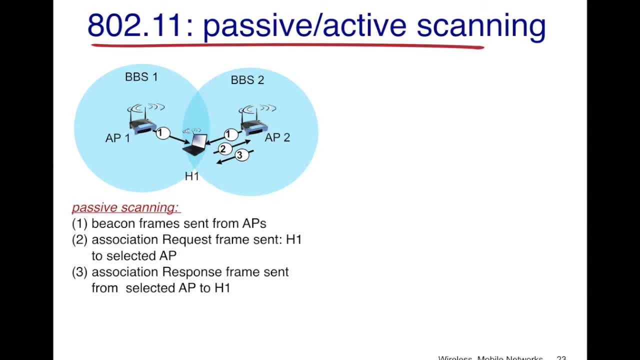 sent from the aps or the access points. now, when a host arrives in, if you, if you look at the figure, it receives two, uh two beacons, and that is marked as one from access point one and from access point two. now this host then has to choose which access point it wants to connect to. typically, hosts 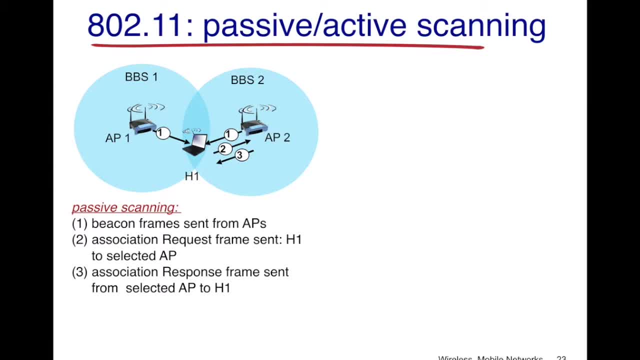 would connect to that access point to which they have the best signal quality, so that they have better data rates. so let's assume that access point two has better signal quality than uh access point one and hence host one connects to access point two. so to do that what it does it. 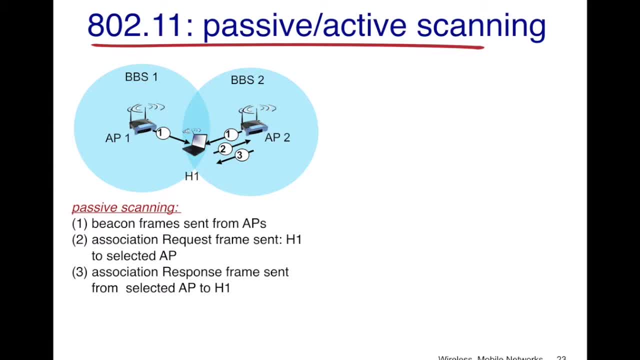 sends a request, association request message, which is in mouth as two in that figure, and once the access point receives this association request message, it sends a response saying that you have, you have now been connected to this access point. this is what happens in path- a passive scanning, now in active scanning and the the opposite methodology occurs. so when a 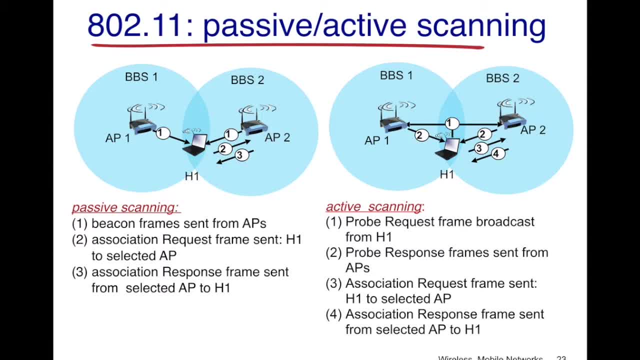 host enters into a network, it sends out this broadcast message saying that it is here and it wants to connect to this wi-fi network. now all the access points which are in this message typically reply back to the host. so in this figure, if you see in the first, 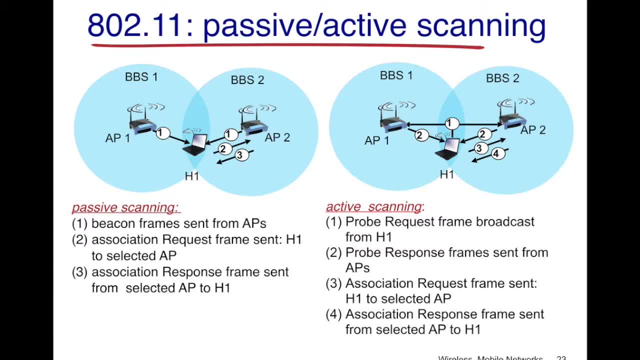 step. the host one is sending out the broadcast message which reaches both access point one and access point two. both access points one and two respond and and they send a response message. now, once the host receives these response messages, what it does is it's typically chooses once again. 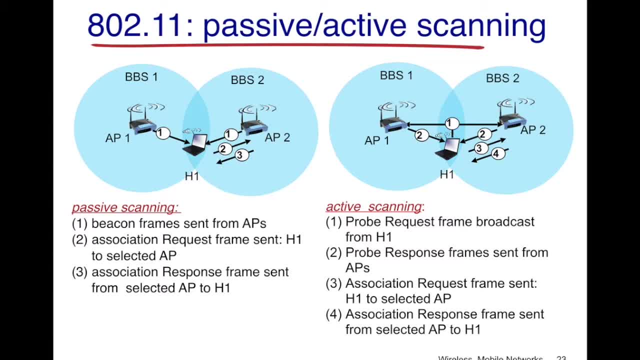 the y, the access point from which it has the, to which it has the best signal quality, and it's sent to the host and it sends the association request. that's what happens in step three and then in step four, the ap says that it is uh that they, they are connected and that the host can send. 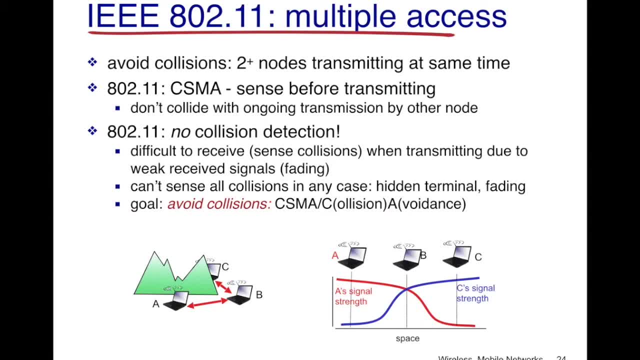 messages to the greater internet through the ap. now, the next important aspect of a22.11 is multiple access. now, in your home network itself, you would have seen that there are multiple devices which are connected at the same time. that is your wi-fi router. now all these devices are using a shared 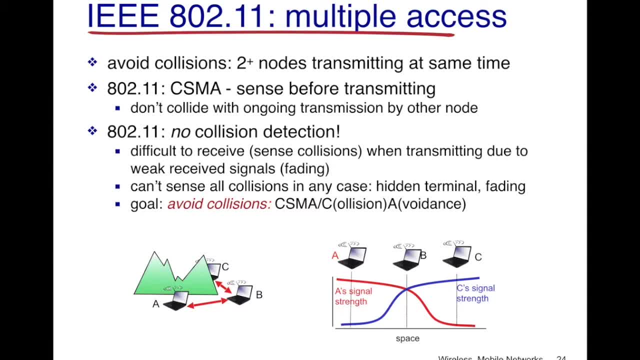 medium which is wireless. now, what happens when multiple nodes communicate with each other over a wireless medium? now when, if multiple nodes communicate at the same time or they transmit at the same time, what can happen is there can be collisions. this is to give you a good example. 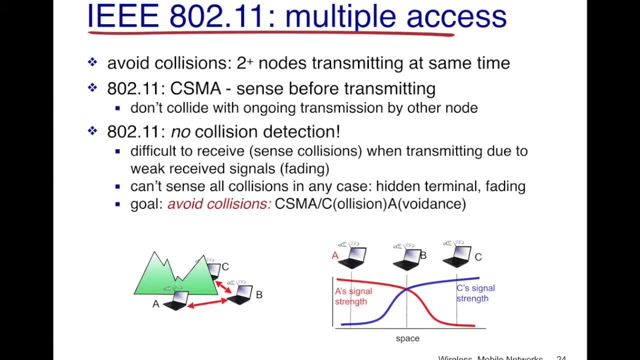 if two people talk at the same time, it is very difficult to understand what each of them is individually saying. this is because their words are colliding with each other. so the why these kind of collisions. what is typically used is csma. now what is csma, csma? 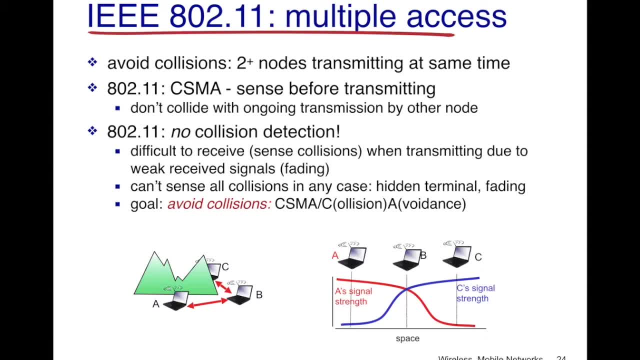 is the acronym for career sense, multiple access- and it's basic. what it incorporates is basic common sense. that is, before a node transmits, what it checks is: is there an ongoing transmission? if there is an ongoing transmission, it does not make any sense for this node to transmit because 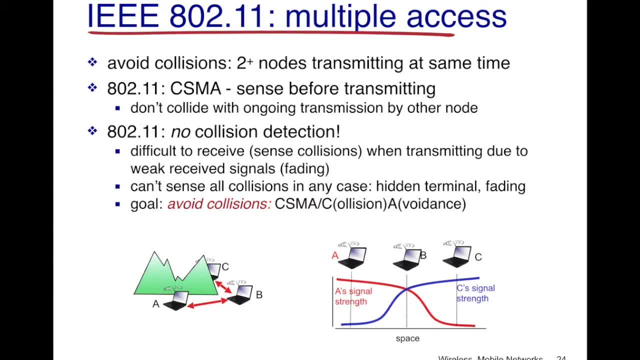 then what is going to happen is the ongoing transmission is also going to get corrupted, so it just keeps silent if there is an ongoing transmission, but then what it does is, if there is no ongoing transmission, it can then transmit. but the biggest issue is that- see this just having. 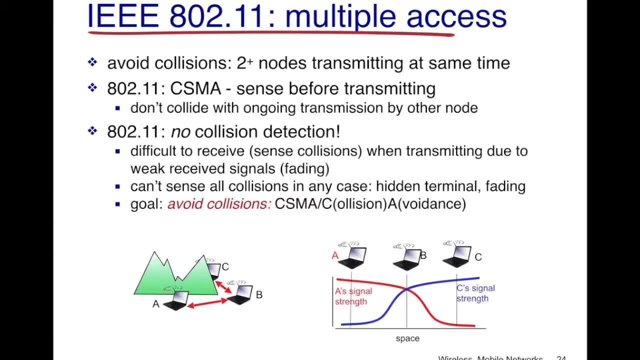 csma is not sufficient because in a wireless network there is no way to detect a collision. this is because signal is very difficult to receive and they are weak, weakened due to a whole bunch of factors that happen in the environment and hence the the receivers are not well equipped to detect. 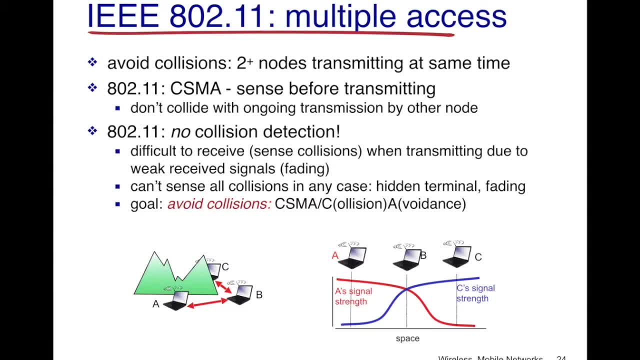 collisions. so how, what would a node do if it cannot detect a collision? say, a collision happened and the node does not even know that a collision has happened, then it wouldn't even transmit the same packet again, and this is not acceptable. so to do that, the goal is to have avoidance, which is 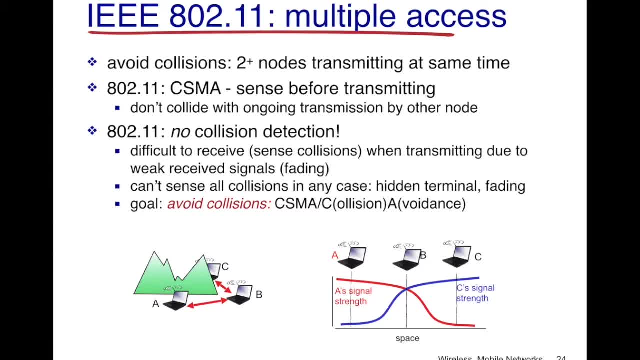 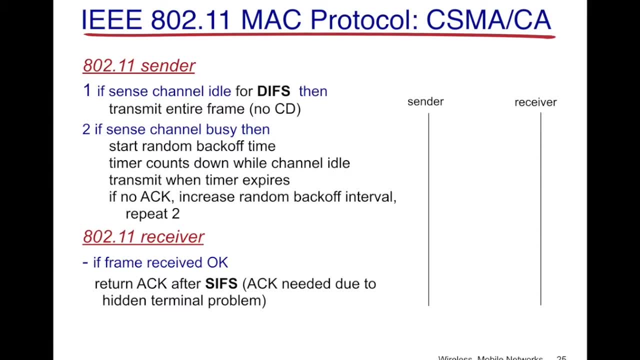 see it, and the protocol is csma ca, where ca stands for collision avoidance. so let's try to understand this particular multiple access protocol. so in csv ca, what the 822.11 sender does is if the channel is idle for a diffs, which is a small period of time. 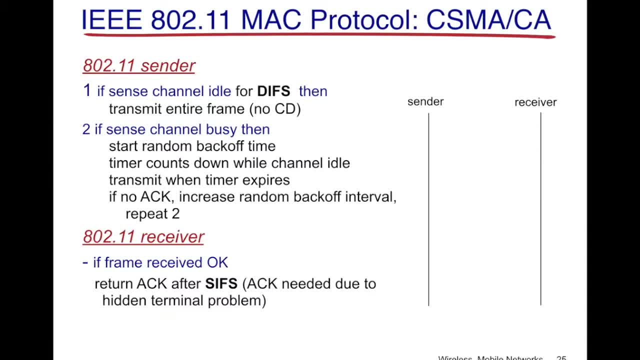 for which it senses the channel, then it can transmit the entire frame. now, if the channel is busy, what it would do is it would back off for a certain period of time and then check again to see if the channel is idle. okay, now at the receiver, if the pre, if the frame is received, 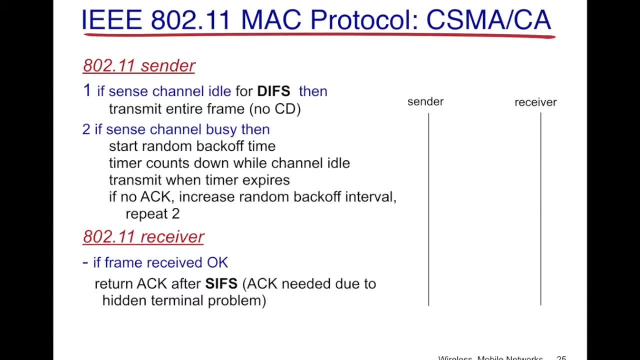 correctly. what it would do is it would return an acknowledgement after a sips, which is another short duration of time and just to make sure that no collisions occur. so let's just see how this protocol works. so first the sender waits for the diffs and then it sends the data. the receiver waits. 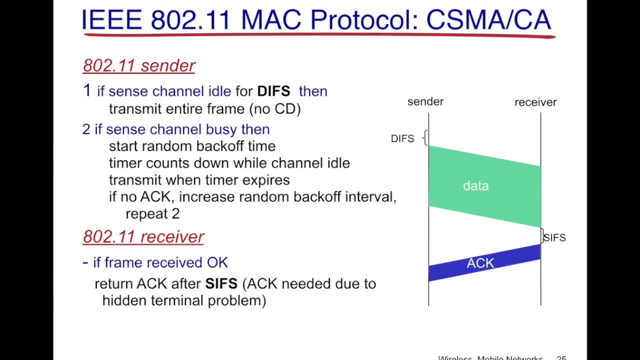 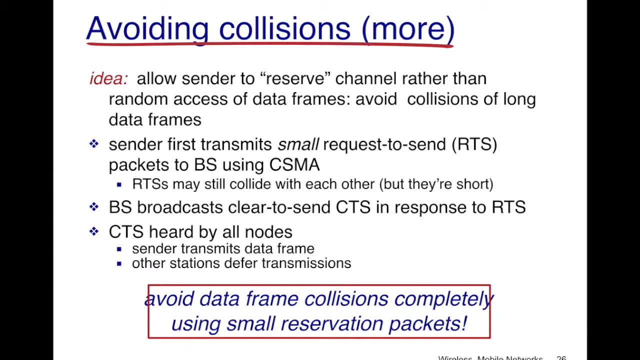 for a small period of time, which is equivalent to sips, before sending back the acknowledgement. now let's try to understand a little bit more about what happens, how collisions are avoided in this case. now, to prevent collisions from happening, what 822.11 allows us is to use 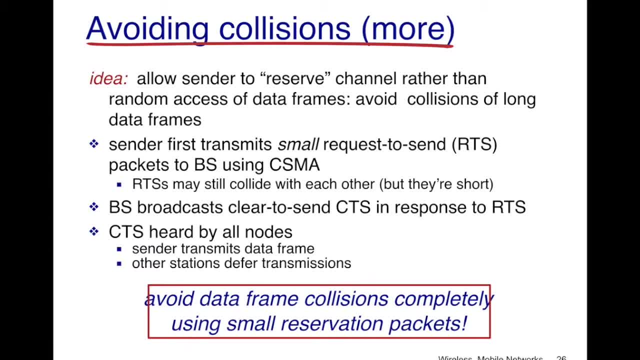 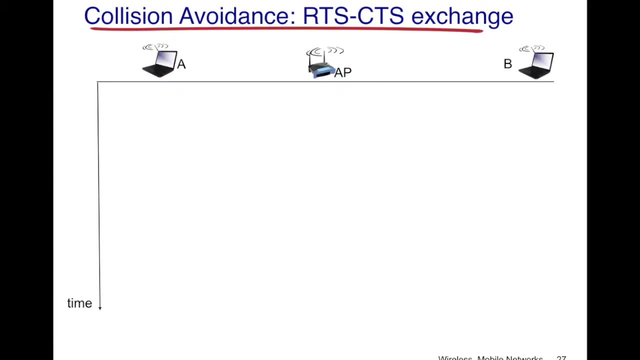 something called rts cts. now rts is request to transmit, while cts is a clear to clear to send. now the basic idea is for a host to reserve the channel before sending its data so that collisions can be avoided. so let's see how this rts ct is actually works. so let's assume that 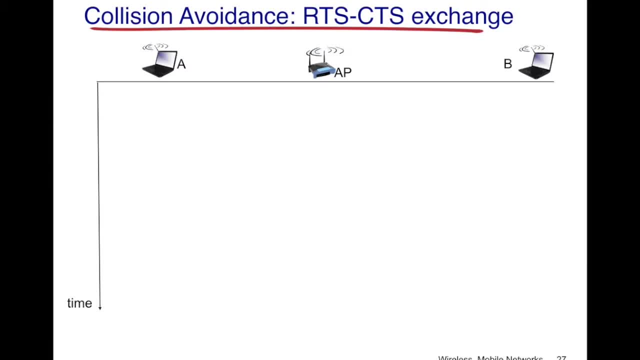 this is the scenario where there are hosts a and b and there is an point in between. What host A and host D want to do is they both have data that they want to send. So the first, before sending the data, they want to reserve the channel. So let's assume that both host A and host B send this RTS. 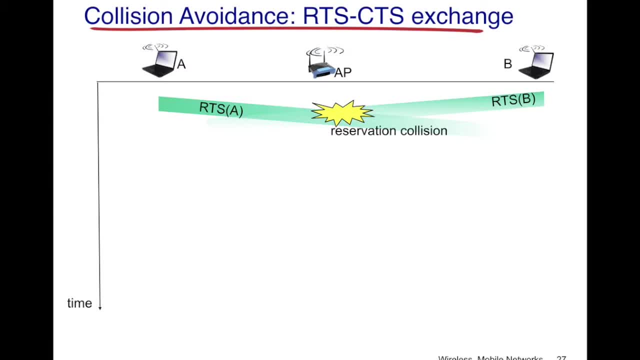 Happens that there is a collision because they both transmitted at the same time and the AP cannot decode the messages that were sent by A and B. After this, both of them wait for some time, and let's assume that the host A then transmits the RTS again, and this time host B is not sending the RTS. Now what? 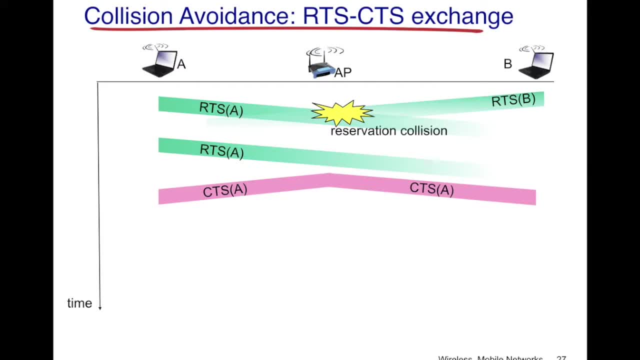 happens is the AP receives this RTS and if you follow the green bar you can see that it's slowly fading. So what it signifies is this RTS message sent by A does not reach B, So B is not aware of the fact that A has actually sent a request to send Now, when the access 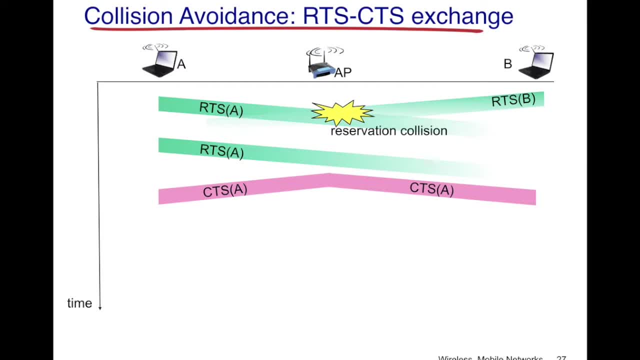 point receives it. what it sends is this CT message saying that is A is clear to send. This message is received by both A and B. Now B knows, because it receives a CT for A, that it knows that A has the channel and he would refrain. 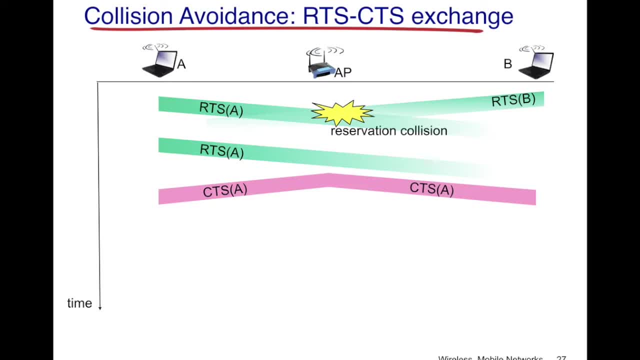 from sending its RTS, which is, it wants to have the channel until A is transmitting. So now, after this, A has the channel, so it transmits the entire data, and after the data has been transmitted to the access point, what the access point does, is it basically? 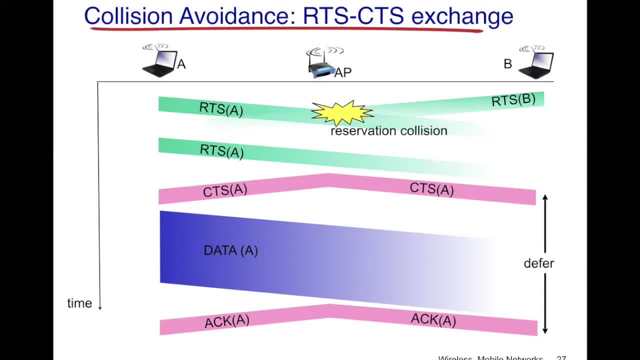 sends an acknowledgement saying that the data has been correctly received. Now, after this, B is now free to send another RTS message to get hold of the channel again. So this is how RTS-CTS works in CSMA-CA and, with the use of this, RTS and CTS collision. 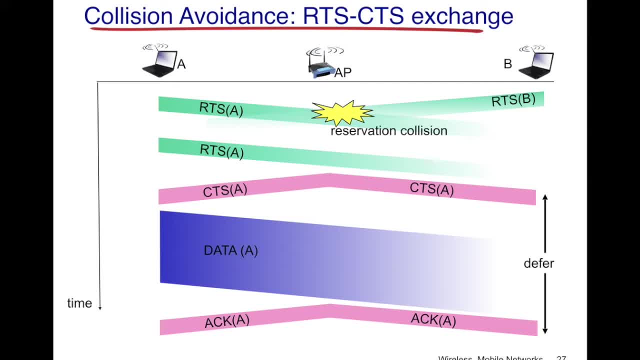 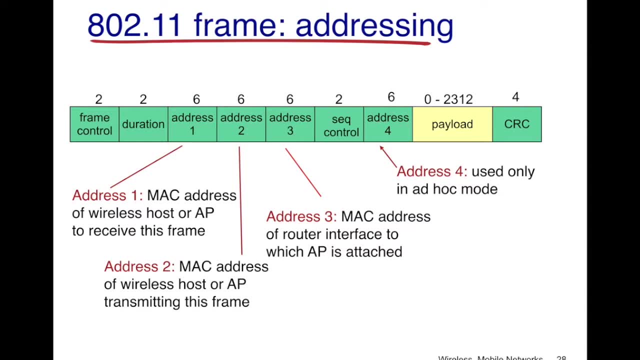 avoidance is ensured in an A22.11 network. There's a last thing that I want to talk to you about. in A22.11 is addressing. Now, in an Ethernet, if you remember, there were only two MAC addresses, But here in A22.11, there were only two MAC addresses. 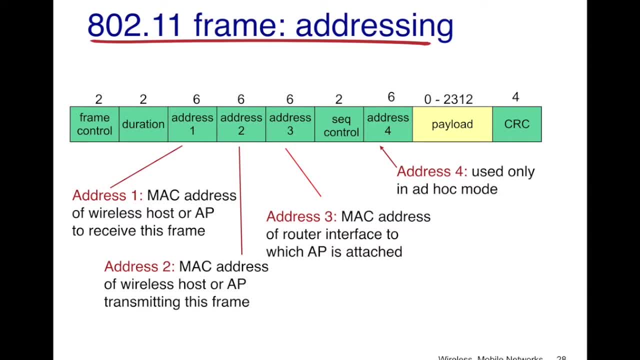 The first address is the MAC address of the wireless host or access point which is about to receive this frame, and the second address is the MAC address of the wireless host or AP which is transmitting the frame. and the third is the MAC address of the router interface. 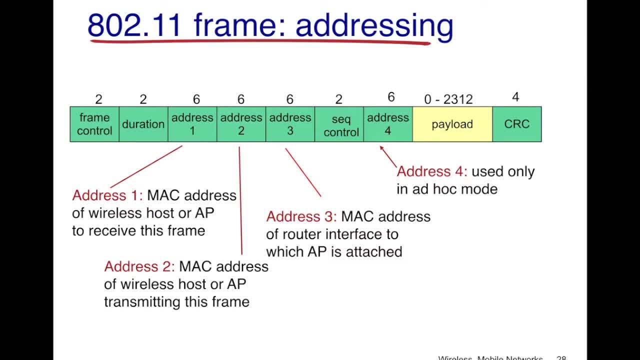 to which the AP is attached. So let's see why we need these three addresses in an A22.11 frame, whereas in an A22.11, that is, Ethernet- we only required two addresses. So let's look at this particular example. 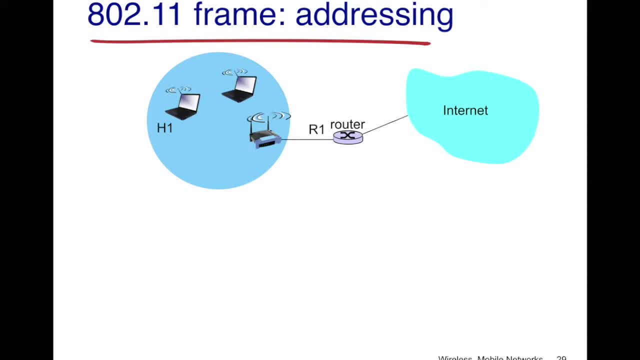 So now host A is sending a frame, sorry, host H1 is sending a frame. So what happens is in the first address it has the address of the AP, the second is its own address, which is H1's MAC address, and in address three is the MAC address of the. 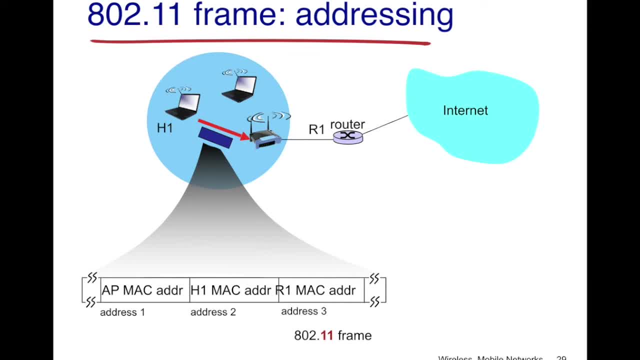 router. now H1 is going to communicate with the router R1 using this access point. Now the router is connected using a wired link to the access point, whereas the link between H1 and access point is wireless. So there is A22.11 technology in the wireless link and there is Ethernet on the wired link.